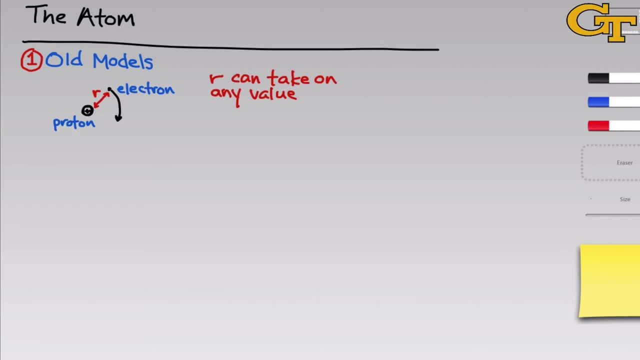 there And if that value r can vary continuously and take on any value, that means that we should expect a continuous spectrum of energies for the atom. Depending on the distance r, we could achieve any energy that we wanted In terms of the light emitted by the atom. 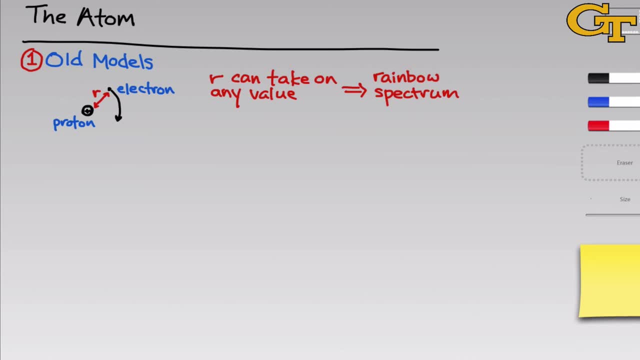 this implies a rainbow spectrum. as we will shortly see, energy is inversely proportional to wavelength, And so if we can get any energy value, we should be able to get any wavelength of light out of the atom, and if we give it enough energy, we ought to observe a rainbow of colors. 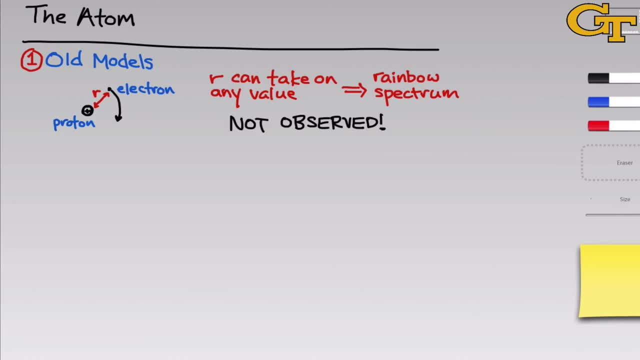 emitted by the atom. However, this is not what observed in practice. Instead of observing a rainbow, we only observe the emission of very specific wavelengths of light from the atom, So we see very thin lines instead of a continuous rainbow of colors. According to quantum mechanics, the wavelength is inversely proportional to the 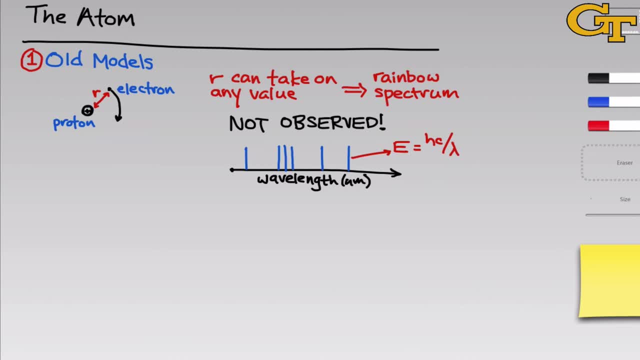 energy. Namely, the energy is equal to h, a constant called Planck's constant times, the speed of light divided by the wavelength. This can also be written as h times nu, where nu is the frequency of the light. So this seems a little bit strange. Instead of r being able to take on 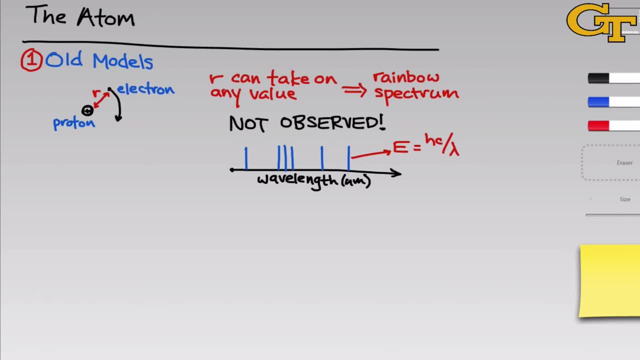 any old value. it appears that r can only assume very specific values. The electron only seems to be able to occupy particular distances from the nucleus. Some new models of the atom were needed to explain this, and the first one that really took hold, which was developed by Bohr, used 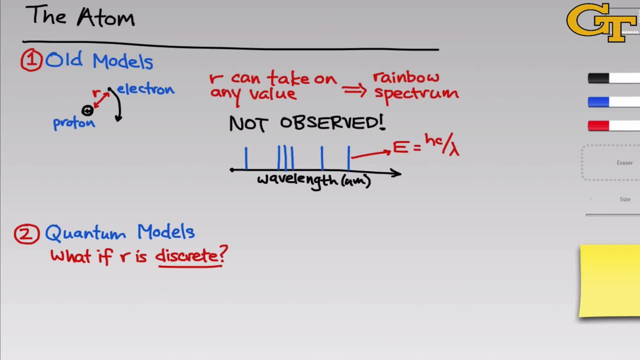 this idea that r cannot be continuous. It can only take on discrete values. Now, and this is a theme we'll come back to again and again, the number of these values may be infinite, So the atom can assume infinite energy, but the important point is that there are finite distances between 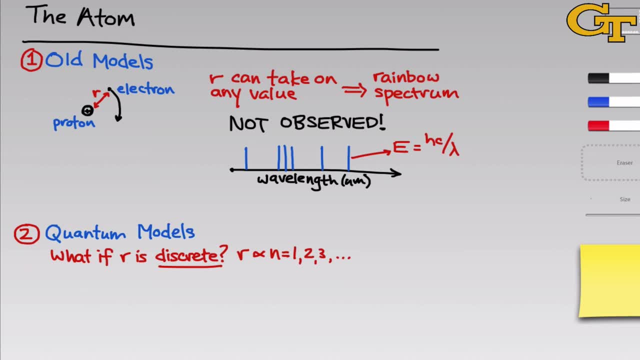 the possible r values. So r is proportional then to something like an integer n. That's one, two, three, four. Notice there's a finite difference between those n values. They have to be integers, so r can only assume very specific values. However, that number